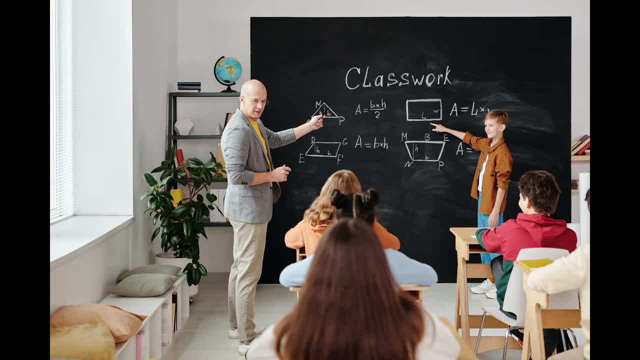 steps forward. The class keeps asking the question until the wolf answers. The wolf says it's dinner time, at which point he turns around and tries to catch someone. The person he catches then becomes the wolf for the next round. Telephone. Split the class into two teams. Have students stand or sit in a line and whisper a. 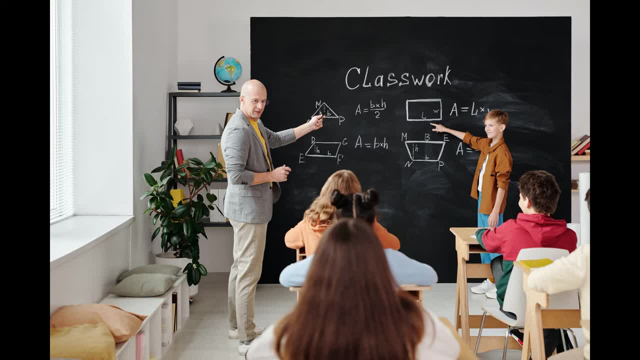 sentence to the first student. Each student then whispers what they heard to the next student until they get to the end of the line. The last student then says the sentence aloud. The team who is closest to the original sentence wins Basketball Using an empty waste paper bin as the basket and a screwed up piece of paper as the ball. 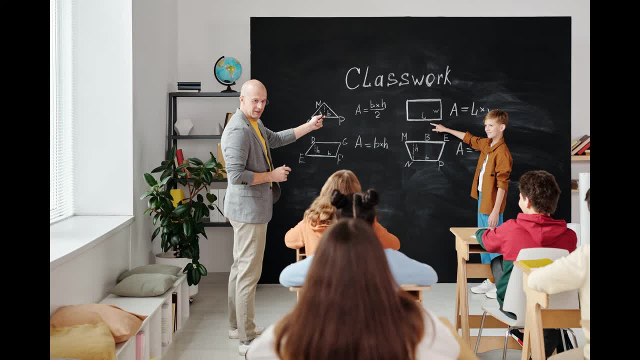 the students have to try and throw the ball into the basket Before they can take their shot. they must answer a question from the teacher correctly. If they get the ball in the basket, they get two points. If they hit the basket but don't get the ball in, they get one point. 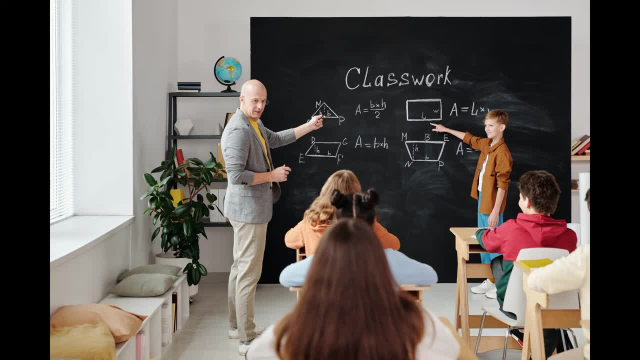 Volleyball. Use two chairs and a piece of string to make a net across the middle of the classroom and use a balloon as the ball. Divide the class into two teams and have them play volleyball. When a winning shot is played, the teacher asks the whole class a question. The team that answers 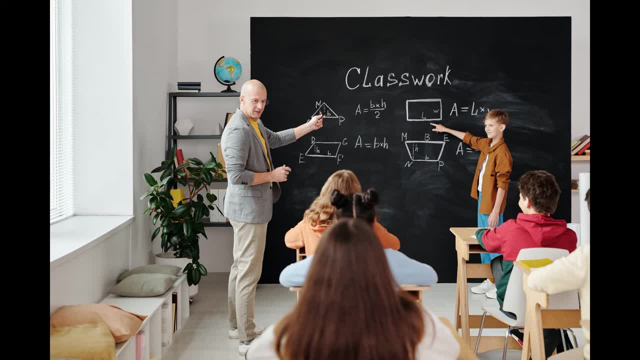 correctly wins the point and gets to serve next Bingo. This classic game can be played with numbers, words or pictures on the students' bingo cards. The teacher calls out a number or word and the students mark off the corresponding number or word on their card. The first person to complete. 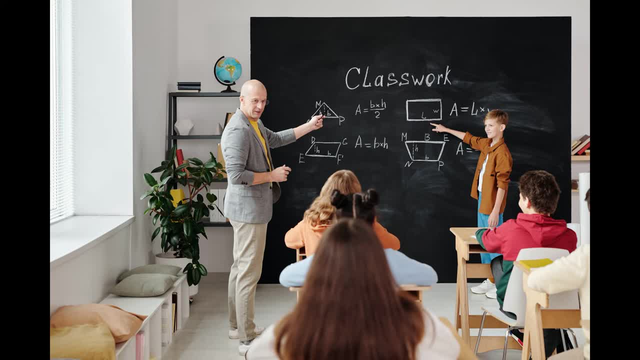 their card, shouts out bingo and wins the round. Can you? The teacher asks students if they can do certain actions. If they can, the student answers yes, I can, and then performs the action. If they can't, they say no, I can. and the teacher asks them if they can do another action. 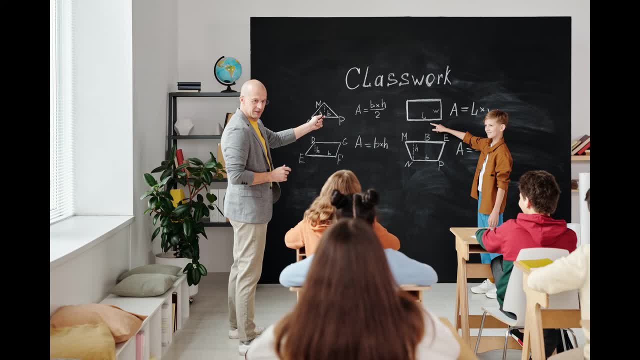 Be sure to have some actions that are easy for shy students to do. for example, can you smile, I spy. The teacher starts the activity by saying I spy with my little eye. something beginning with, and chooses the first letter of the object. Students have to guess what object the teacher. 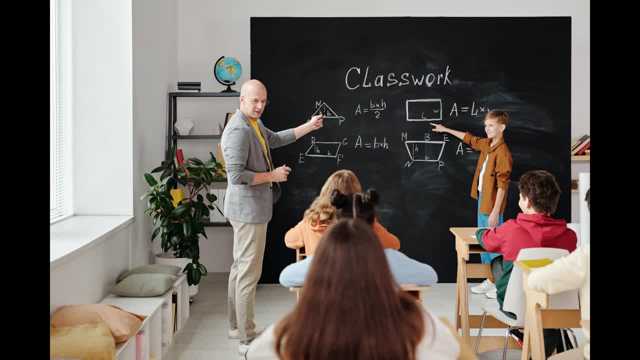 is thinking of. The first letter of the object is the letter of the object If they can do certain actions. the teacher asks them if they can do certain actions. If they can, the student answers yes, I can, and First person to guess correctly takes over the teacher's position. 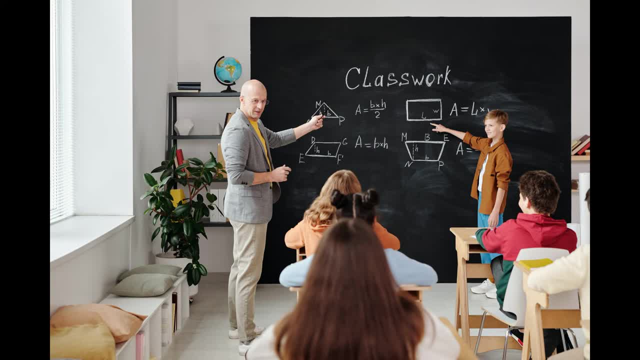 For younger learners, colors can be used instead. for example, I spy with my little eye something that is red. Odd one out. The teacher writes four words on the board, three of which are related to each other in some way, For example, banana, apple, car, strawberry. 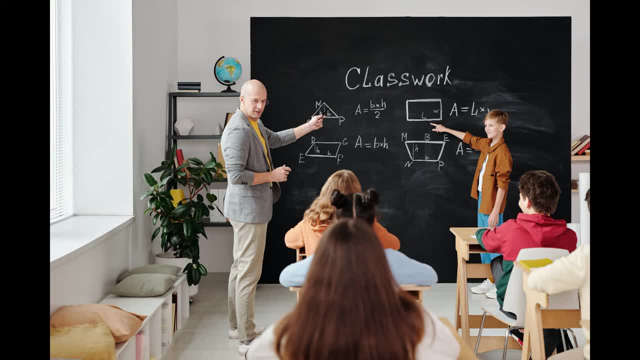 The students have to say which word is the odd one out. This activity can be done with objects or pictures in place of words. Stand up, please A version of Simon says, where the phrase Simon says is replaced with please. The teacher or a student asks the class to do certain actions. 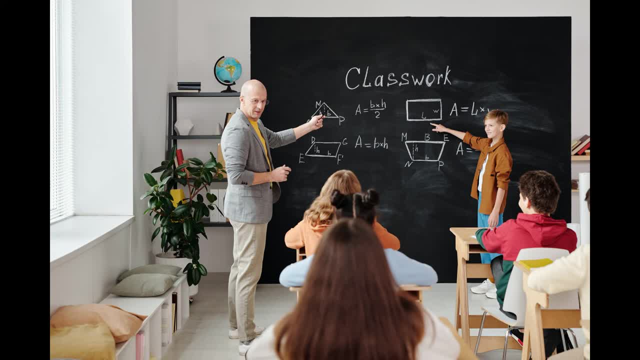 but they must only do them if the teacher says please. Anyone who does the action without please being said is out of the game. Mastermind, This is a good activity for older children. The teacher chooses a four or five letter word and draws the corresponding number of dashes on the board. 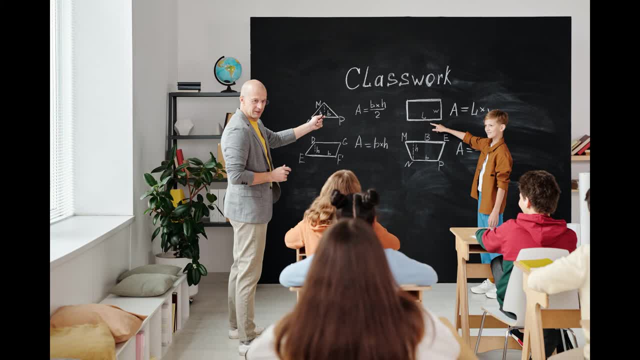 The students have to choose a word of the correct length and one of them writes it on the board. The teacher marks each letter with a tick, a circle or a cross. A tick means the letter is in the original word and is in the same place. 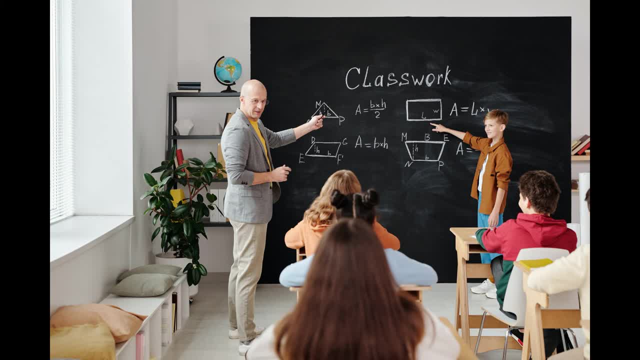 A circle means the letter is in the original word but in the wrong place. A cross means the letter is not in the original word. Blindfold obstacle course. Create a course in the classroom using chairs and desks. Make sure that students won't hurt themselves if they bump into them.